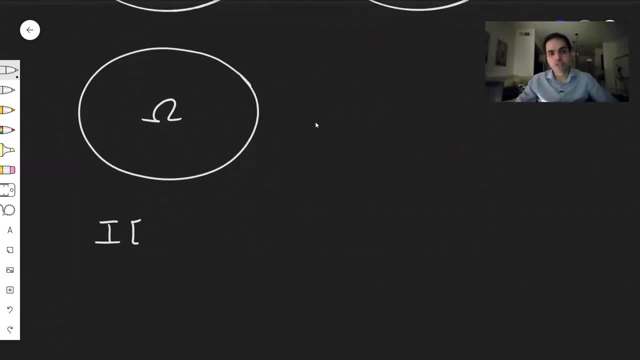 following energy And you're considering the following energy And you're considering the following energy on omega. Let's call it I of u, where u is a function on that domain And what I spits out it's called the energy functional. It's simply the integral over that domain of. 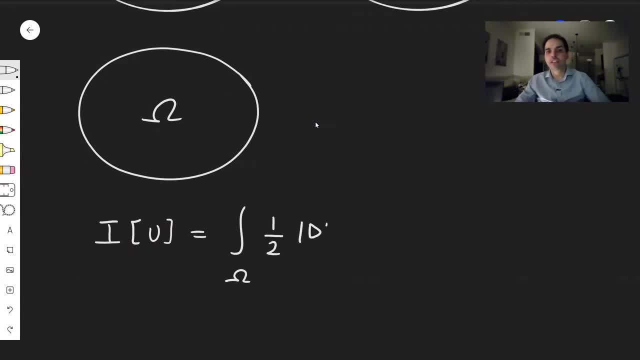 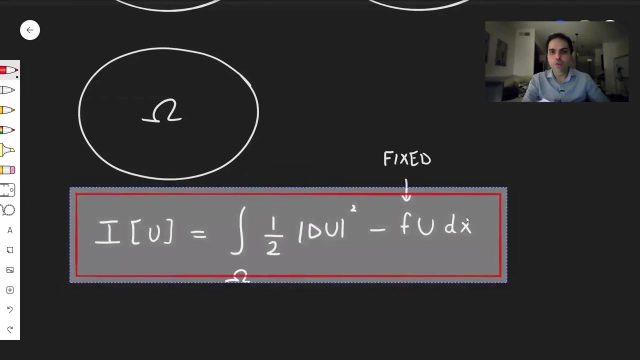 one-half times the length of the derivative squared. one-half du squared minus fu, Just a fixed function f times u function. So this is the functional we'll consider for today, And if you've taken physics you might recognize this actually as something very interesting, because one-half du squared 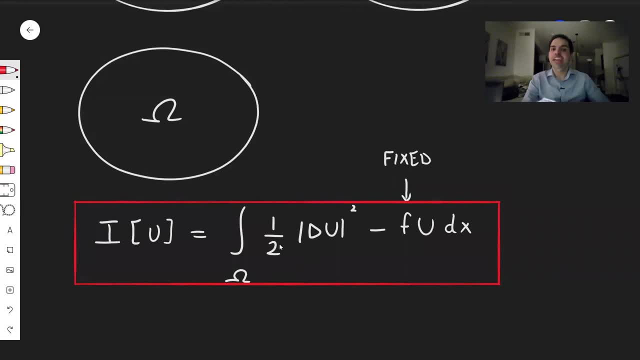 that's nothing other than the kinetic energy. So this is the kinetic energy and this is the potential energy of your system, And what I of u gives you is the total energy of your system. So in calculus of variations, as I said, you connect energies with PDEs, And so this is our energy. 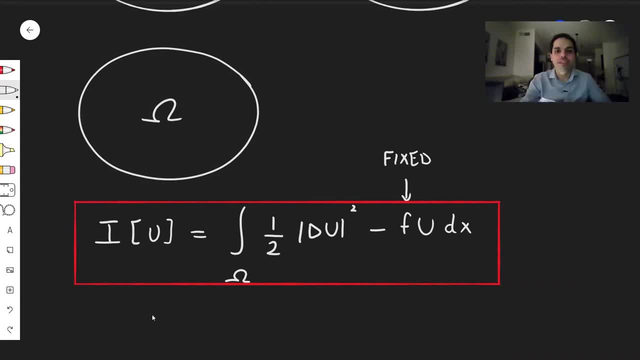 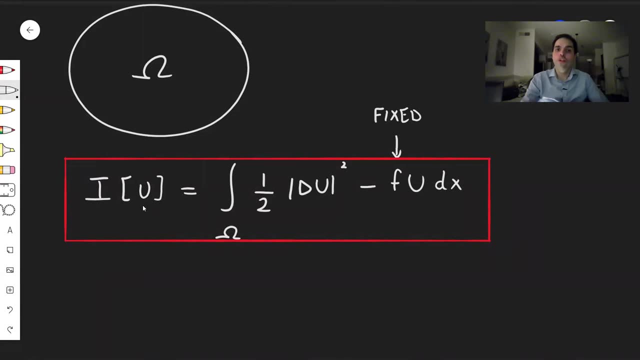 And later we would like to ask what is the corresponding PDE? And that said, though, notice, in this functional we can't just plug in a random function. u, For instance, if you put an absolute value, this doesn't work, So we need to. 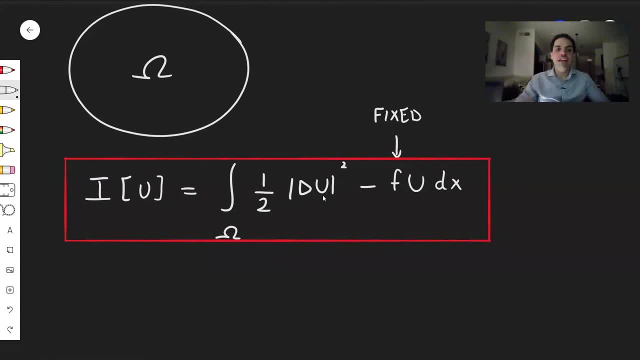 break this down into a small size. Let's look at our functional u. What do we need? We need to talk about a very specific class of functions called the admissible class, MathCal a, And what it is is just the set of all functions v, which in this case, let's say they're infinitely differentiable. 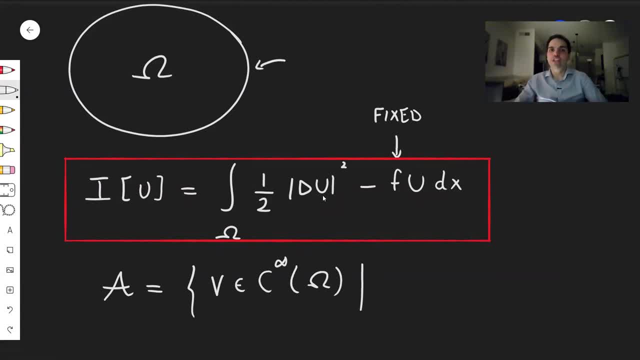 And not only that. let's add a boundary condition. Let's require that our function u equals to some fixed function, u function g. So in other words, the function we're considering are all the smooth functions that are equal to g on the boundary. And now we're ready for the minimization problem. 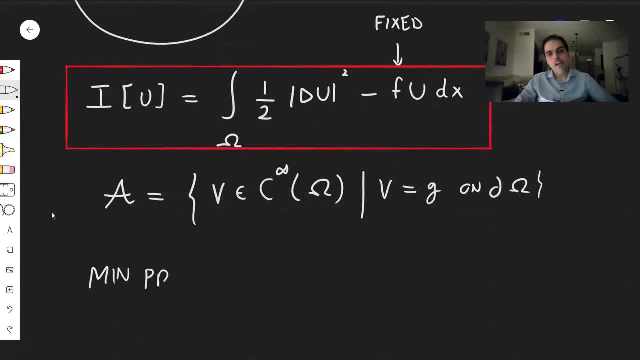 which is the following: Namely, among all the functions v that in this admissible class, so that are infinitely differentiable, with this boundary condition, find the one or the ones that minimizes energy i of u. So, more compactly, what the minimization problem is, just written as: 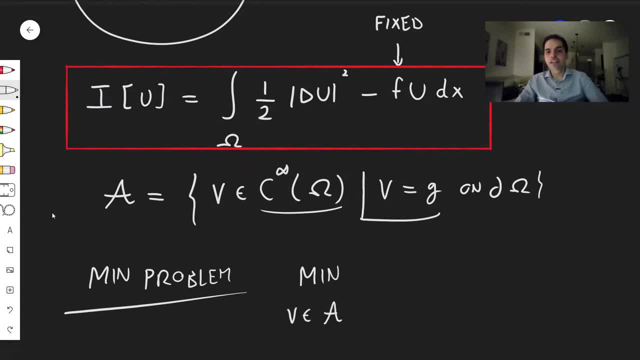 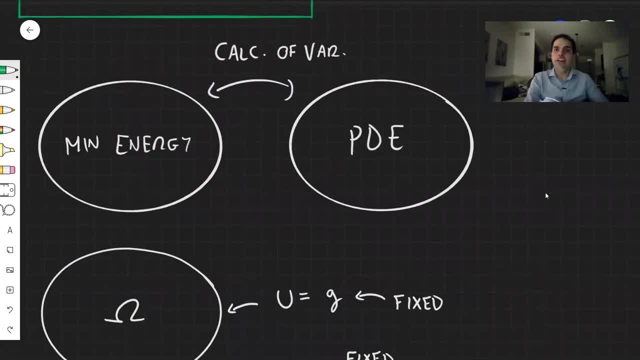 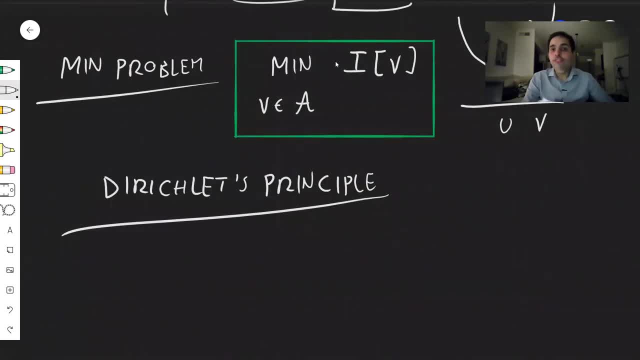 So again we're done now with the energy aspect of the function v, Namely If a function u solves this minimization problem. So suppose u minimizes the energy, so min v and a of I of v, then it turns out it solves a very specific PDE. 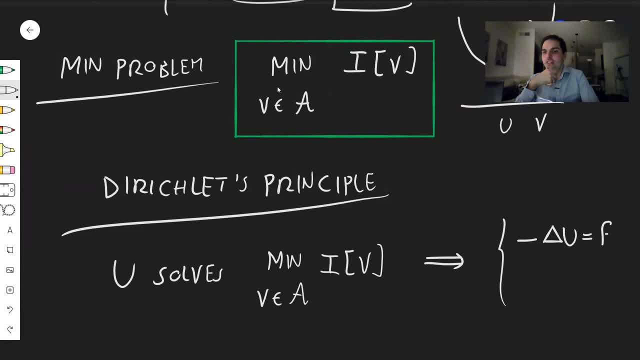 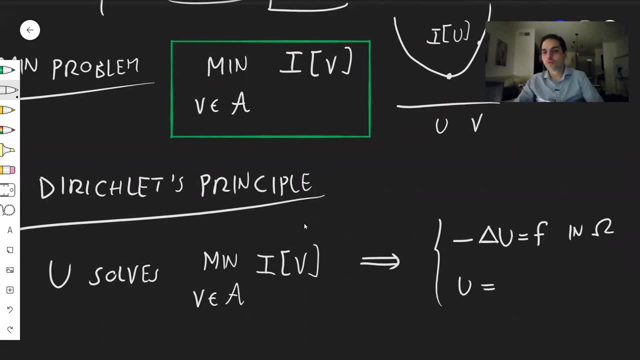 which in this case it's Poisson's equation. So minus Laplace in review equals f in our domain and u equals to g on the boundary, And this is sometimes called the Euler Lagrange equation of this minimization problem. So maybe in another video I will show that, given a minimization, 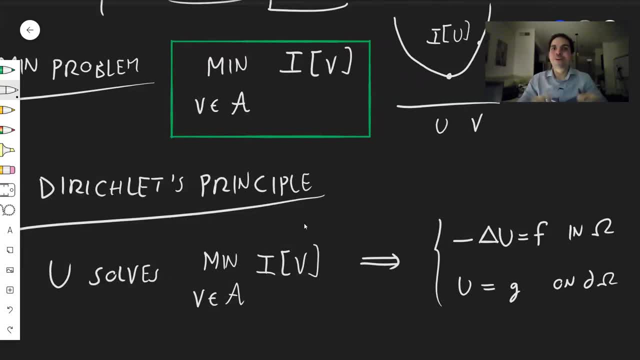 problem. you can extract a PDE from this, But wait, there's more. This is always true, but it turns out in this specific case, the converse is true as well. Namely: u solves this minimization problem if, and only if, it solves the Poisson's equation. And this is what we want to show today, And in fact, 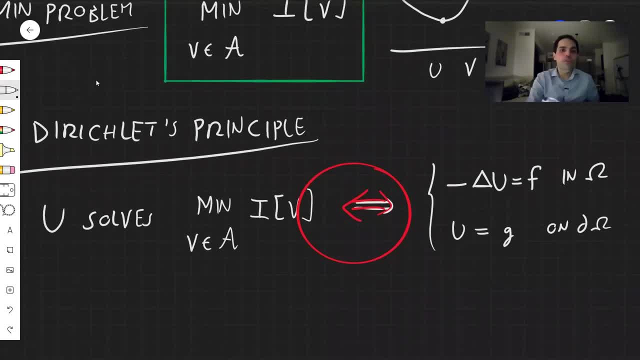 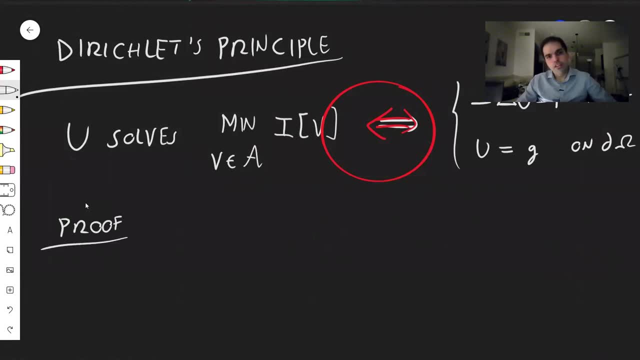 as they say, the proof is in the pudding. So today's pudding is very delicious and this is why I wanted to make the video. So let me prove this. So let's see, Let's do the first part, And the first part is very standard And it's nearly the same proof as the. 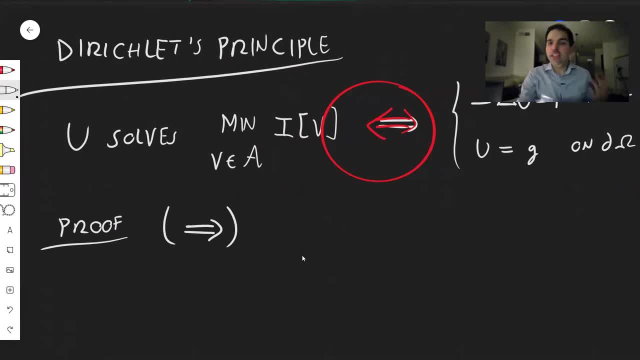 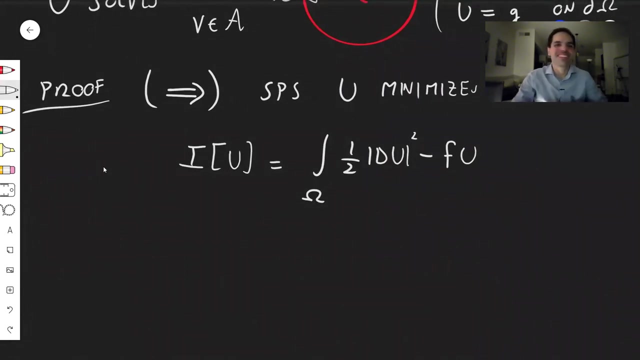 derivation of the Euler Lagrange equations, And it goes as follows: So remember our minimization. So suppose u minimizes, let's say i of u, which is the integral over our domain of one half du squared minus fu. I'm not cursing, It's just f times u All right. So here's the important thing to understand. 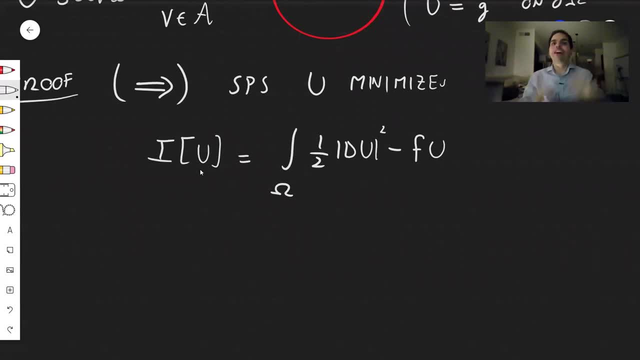 This is functional, Depends on functions. It's very complicated. The beauty of calculus of variations is that we will turn this complicated problem into a single variable calculus problem. So even a Calc 1 student would be able to solve this. How? What I write down now it won't quite make sense, but you'll see in a second why it makes sense. 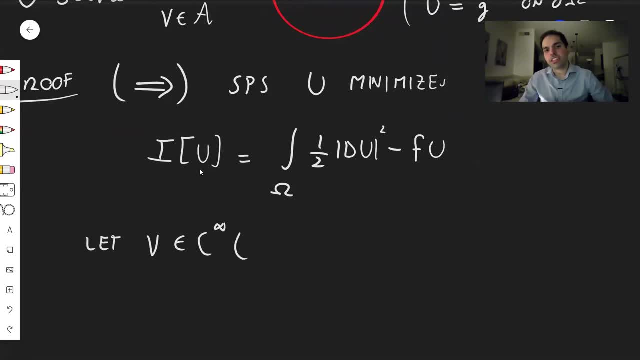 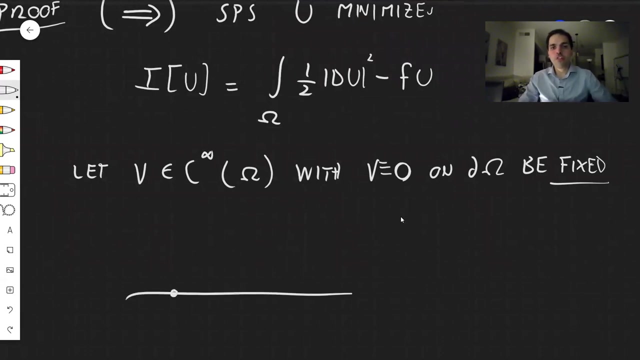 So let v be in c, infinity of omega with v, So with v identically equal to 0 on the boundary, be fixed. We consider an arbitrary function, v, that is 0 on the boundary. So in terms of a profile picture, 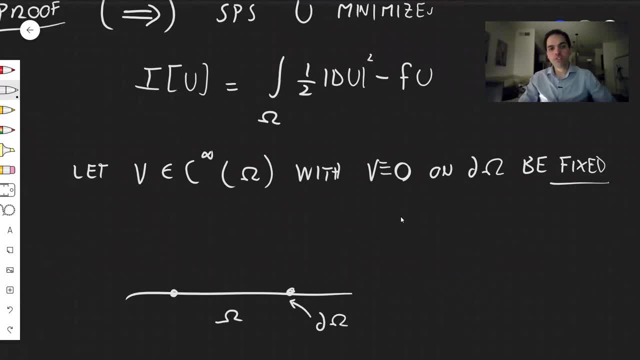 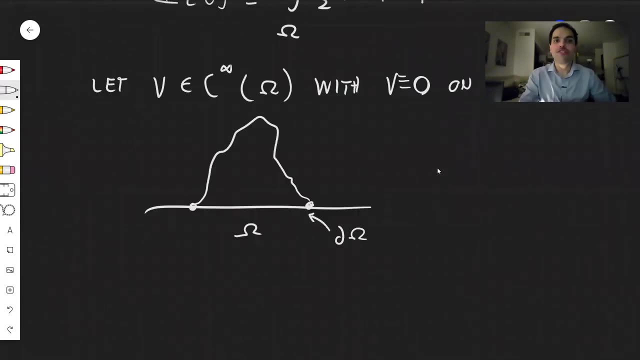 So if this is omega and this is the boundary, what v looks like is just 0 here And then it's whatever in the middle but 0 on the boundary. So again kind of like fixing a web string at 0.. And then consider the following: 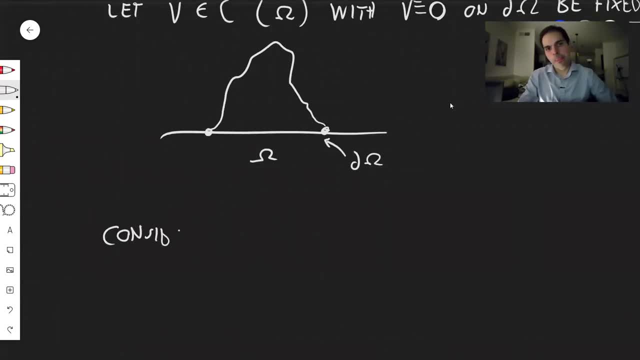 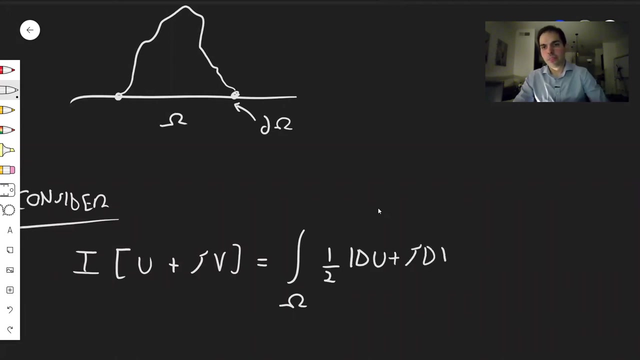 so again, u minimizes our functional v is arbitrary and what we would like to consider is the following: so i, u plus tau v, which is just the following integral over omega of one half d, i think u plus tau dv squared and then minus f times u plus tau v. 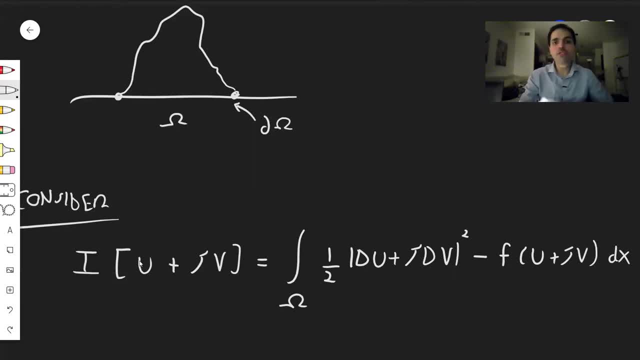 dx, literally replacing u by u plus tau, v and tau. it's not two pi, it's just an arbitrary real number. again i want to emphasize: we know what u is, it's this minimizer. v is an arbitrary function. so u, uv, uv, f is fixed. So really notice this whole thing. all it is, it's just a function. 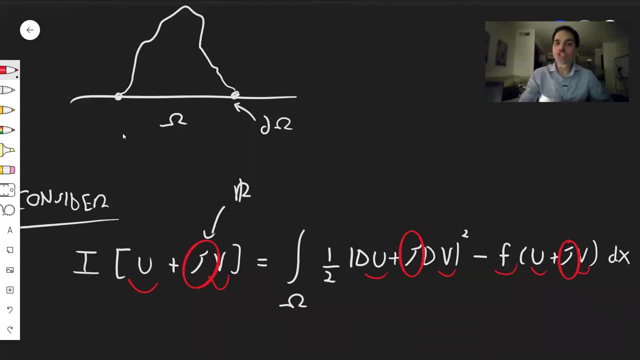 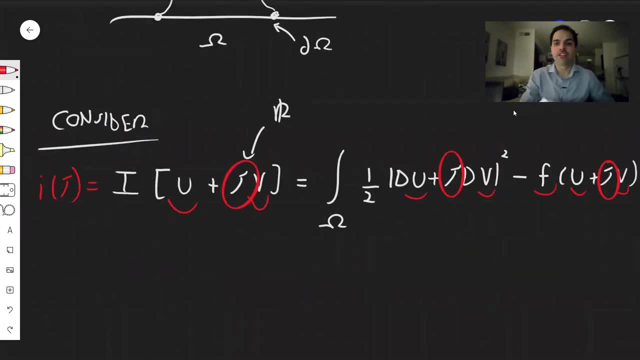 of this variable tau. So it's actually a real function like in calculus And we call this little i of tau. And before I move on, remember there was this admissible class. So we said u was in the admissible class, so u was infinitely differentiable and u is identically equal to g. 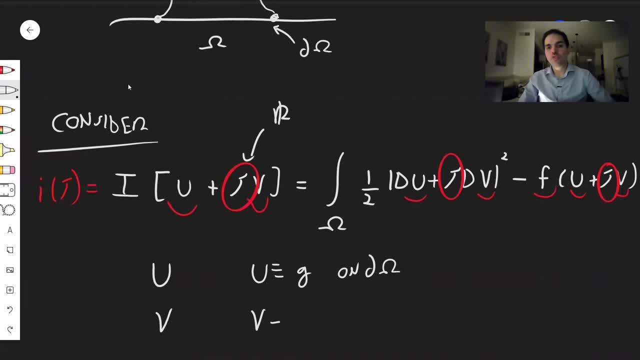 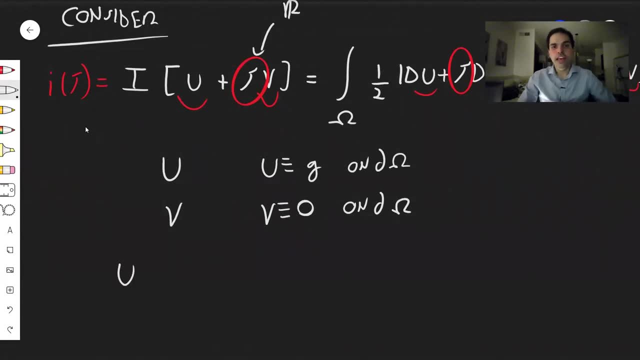 on the boundary And v was defined as just being at zero on the boundary. Well notice, for every tau u plus tau v on the boundary, that's identically equal to g plus tau zero, which is z on the boundary. So in fact, our u plus tau. 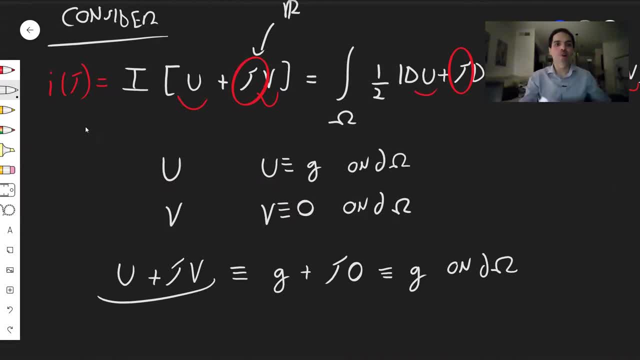 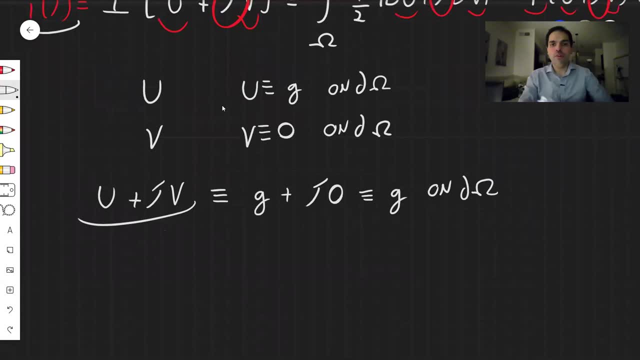 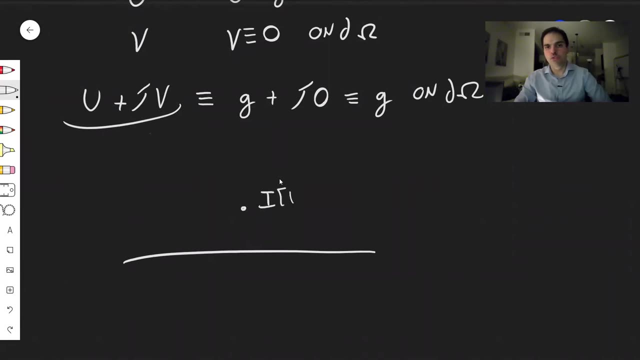 v. they're in our admissible class, They're in the correct class. Now let's look at this function, little i, a little bit more, And remember what we said was this function, this functional, had a minimum at u. So i of u was the minimum, which means for any other function, v it's bigger. 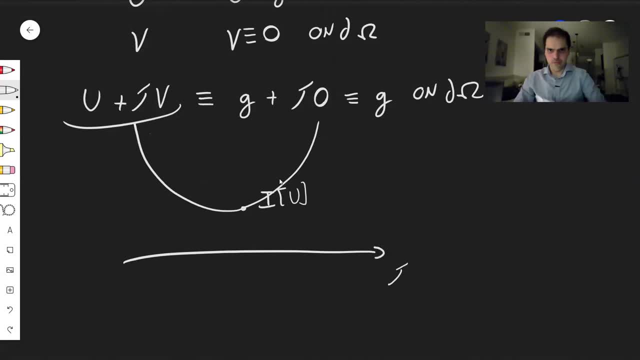 But now let's think of this in terms of tau, or like i of tau. Then if I give you a random tau, then this becomes just the functional of u plus tau v. Now what is this value? Well, it is the same thing as i of u plus zero v. 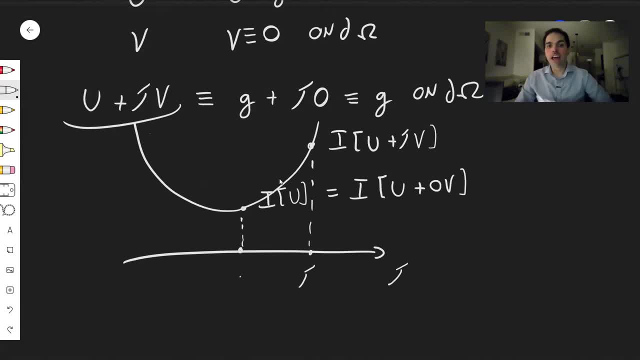 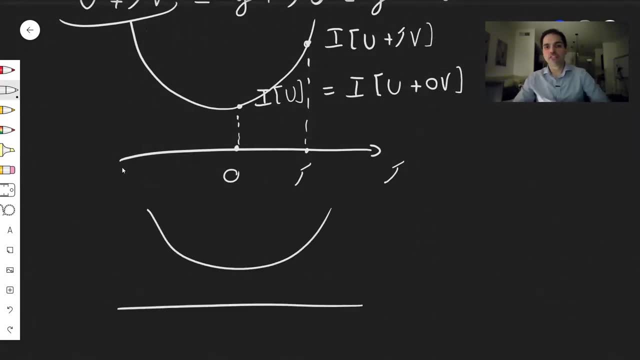 So it's just a value of the little i at zero. So, in other words, if you want to draw the graph of little i, it just looks as follows: So this is tau, This at zero, it is i of zero, And in general for tau, it is i of tau. 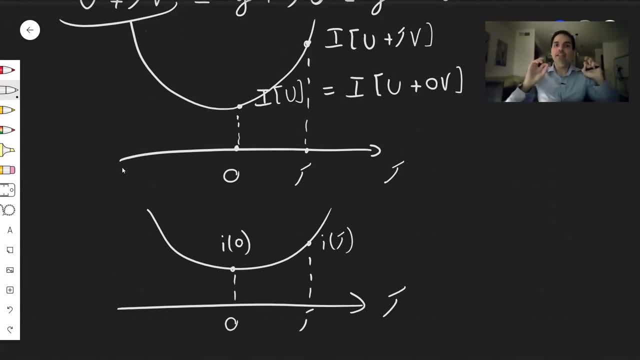 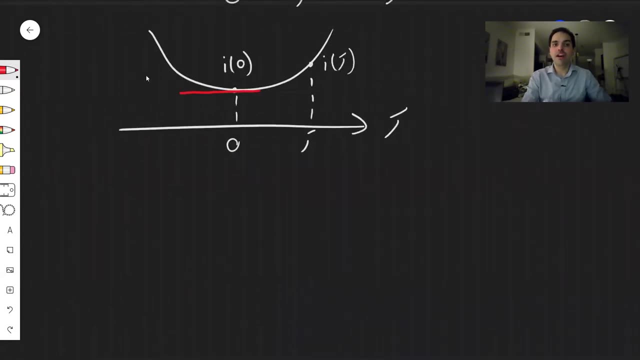 Now I want to emphasize little i, that's a function of one variable. So what do you know from calculus about functions which have minima? Well, by the first derivative test or something, we know that the derivative of little i, i at zero equals zero. And this is what allows us to go from minimizers of functionals to PDEs. 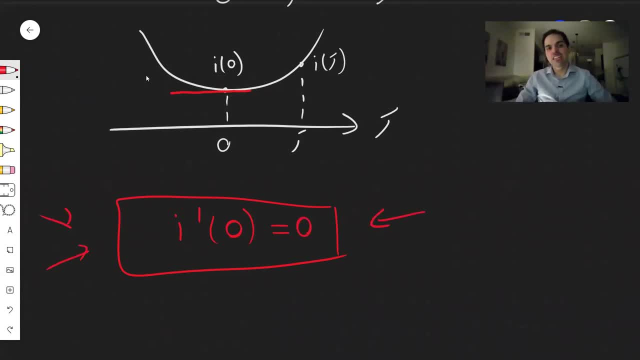 Literally, this is the key to the calculus of variations. Well now the question is: of course this raises a question: what is i prime and what is i prime of zero? Remember, i of tau? that was integral over omega one, half du plus tau dv squared minus f, u plus tau v. 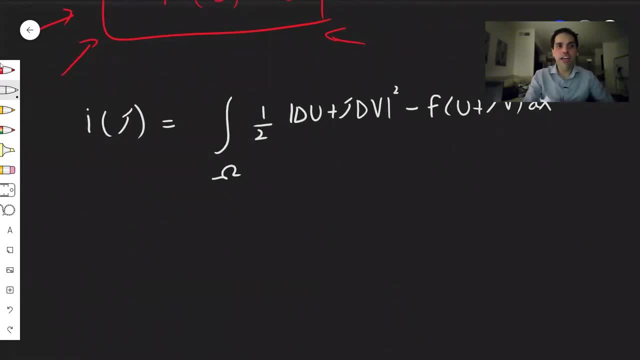 The x is 1.. And well, to differentiate, i well, you just got to use the chain law, so just as usual. So i prime of tau is integral over omega. and then let's see, So one half u is the chain law, so 2 times du plus tau, dv. And then you differentiate this with respect to tau. 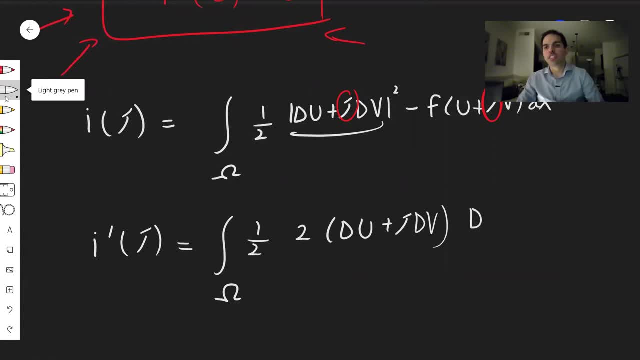 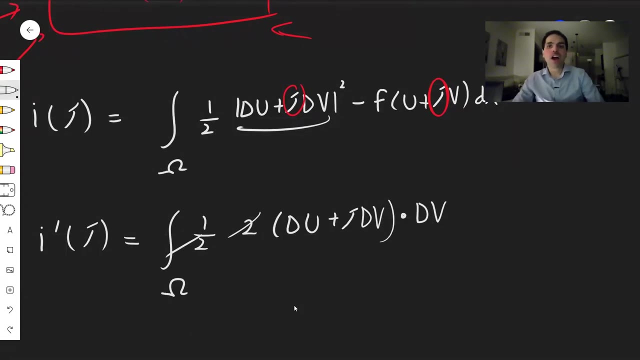 which, again, this is constant- becomes zero and you get dv, dvd, But here we have a vector, here we have a vector. So to make a scalar, you dot it. You can also do it by component, it's fine. And again, this is constant. this is constant with respect to tau. 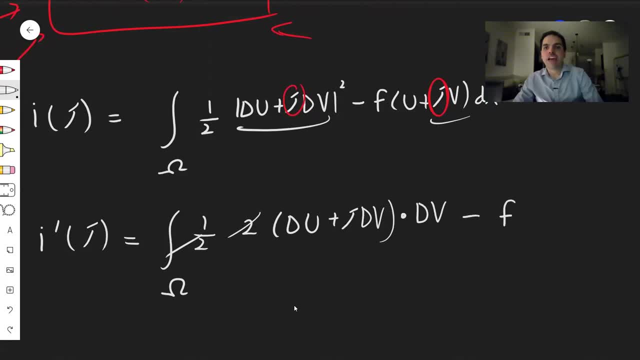 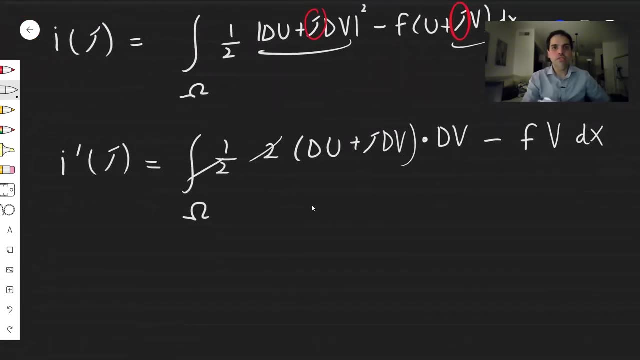 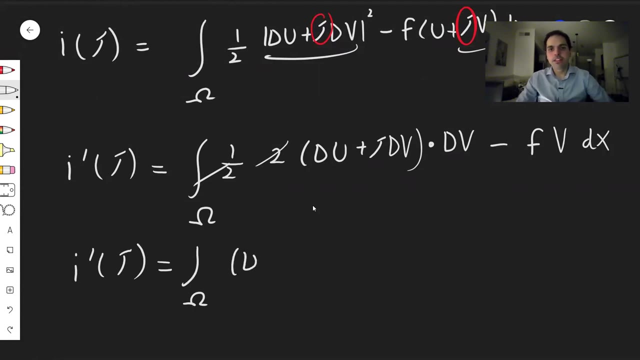 So, really, if you differentiate that, you get minus fv the x, And then what you're left with is simply the following: So i prime of tau is integral over omega du plus tau dv. dot it with dv minus fv the x. 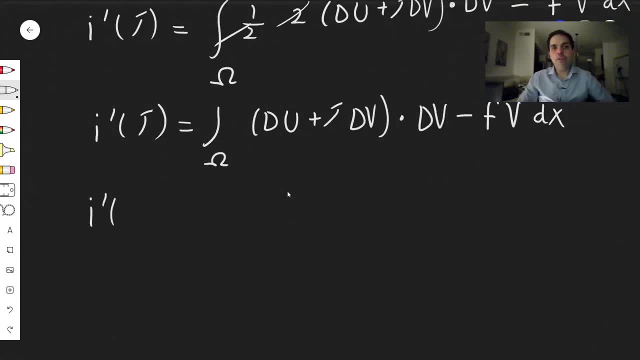 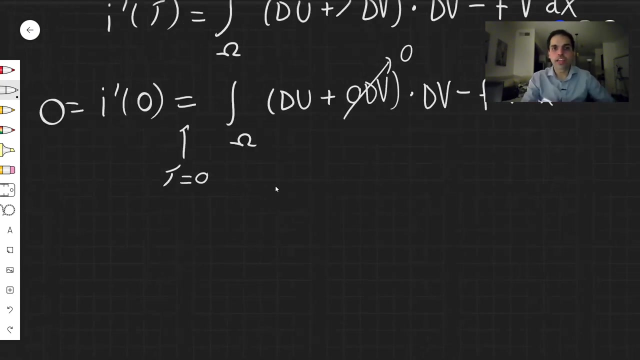 And now we want to use our magic equation, namely i prime of zero. on the one hand, it's zero, on the other hand, you can just let tau be equal to zero here, and you get du plus zero dv, dotted with dv, minus fv, dx. Well, this jumps out and you get 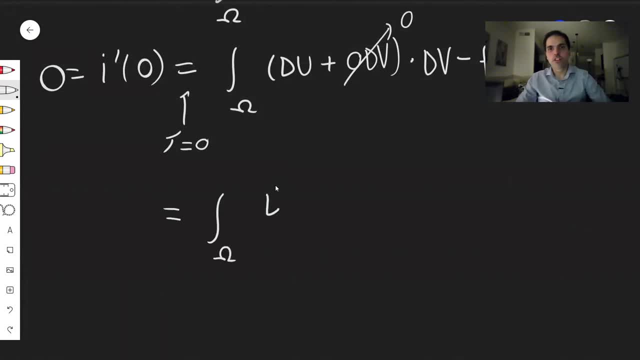 integral of du dotted with dv minus fv, dx. Alright, so what we know is this is zero by assumption. Remember that v is arbitrary and we kind of want to use this. So here we have this derivative. Ideally, we would like to put this derivative here. 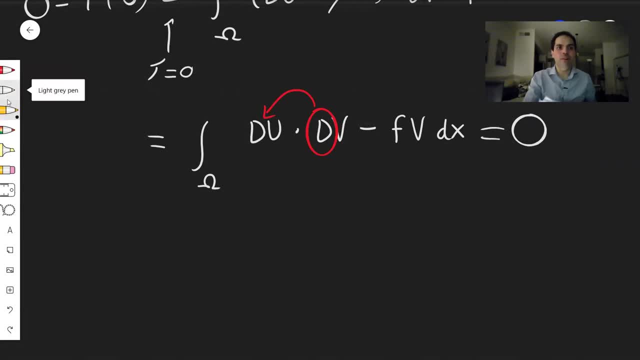 but of course we can simply by integrating by parts. Now, in integration by parts they're usually boundary terms, but not here because, remember, V is zero on the boundary. So yet another reason why we chose V to be zero on the boundary, not only to have U plus tau V. 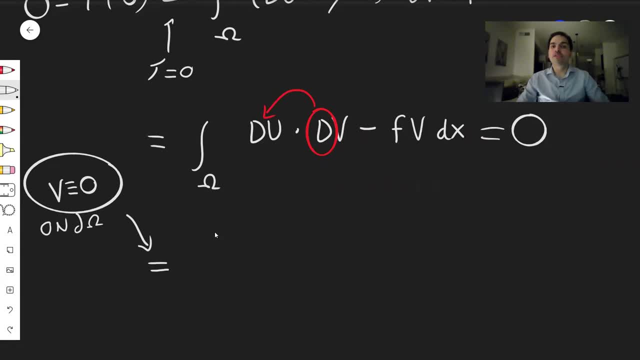 in the admissible class, but also for this integration by parts. So what happens here is that while this D comes here and again, I've done a video on integration by parts and you get, minus Laplacian, U V, minus F, V, dx, which in the end becomes the following integral: 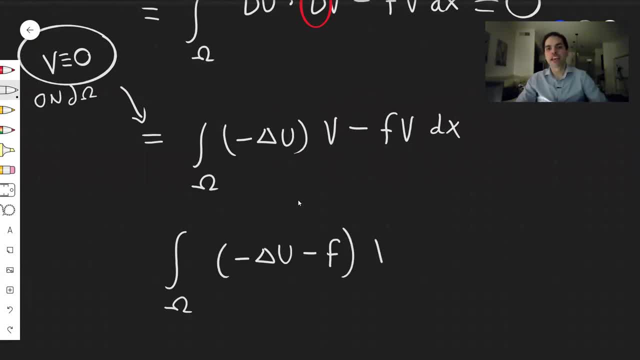 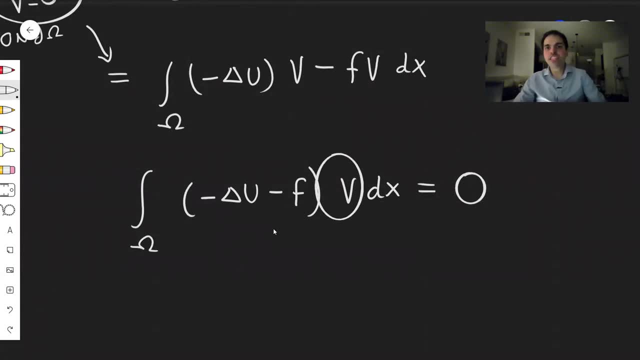 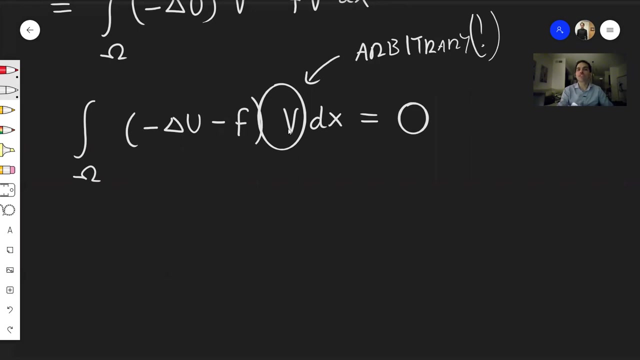 of minus Laplacian, of U minus F, times V, dx equals zero. Now here's the thing: This function V is arbitrary. So just to reiterate, what do we have? We have that for any function V against zero on the boundary. if you integrate this function times V, you get zero. And the question is: what is this? 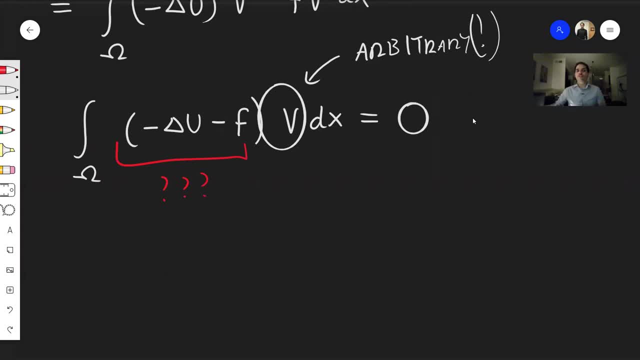 function. So again, suppose I tell you a mystery function, such that, no matter which function you multiply with and integrate, you get zero. Well, the mystery function has to be zero. So what does that mean? Well, the mystery function has to be zero. Well, the mystery function has to be. 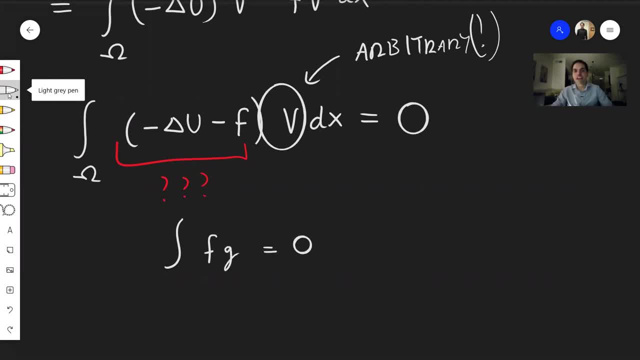 zero. So in other words, I'm using the following fact: If F, G equals zero for all G, then F must be identically equal zero. If you want quick proof of this, suppose it's not zero at a point, then it's, let's say, with our loss of generality, it's positive at the point. Then, if F is continuous, 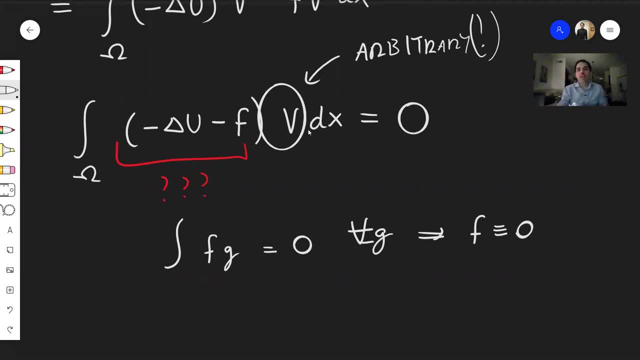 then F is positive on some ball and basically just choose V to be a positive function on that ball, but such that it's not zero. So if F is continuous, then F is positive on some ball, but such that it's not zero. So if F is continuous, then F is positive on some ball, but such that 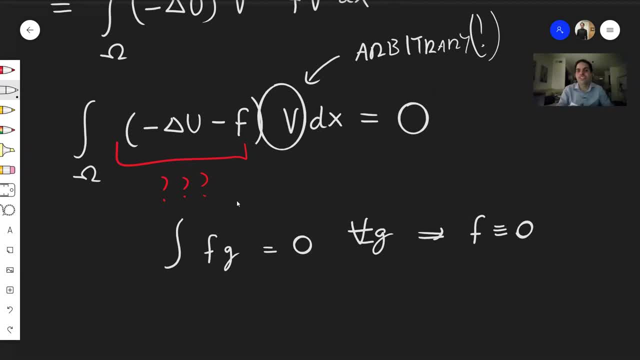 is zero on the boundary. You can do this. It's called a cutoff function And therefore, in the end you get that we get a contradiction. So F must be identically equals zero. So, in particular, what do we get? We get that this inside function is identically equals zero. And what does that? 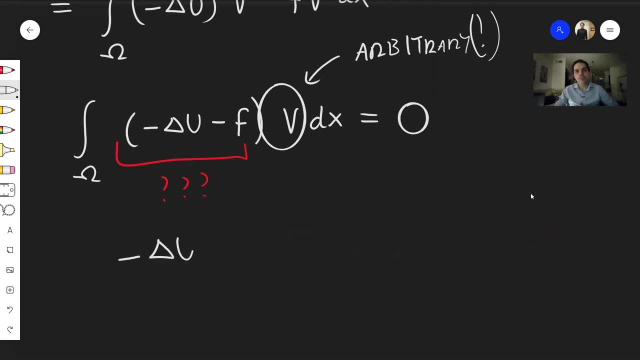 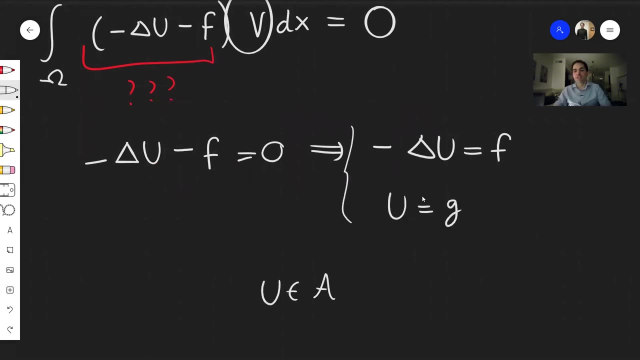 tell us. It tells us that minus Laplacian of U, minus F, equals zero And therefore in the end we get Poisson's equation. and there was also a boundary condition. but remember, U was in the admissible class, so by assumption you always trust G on the boundary. 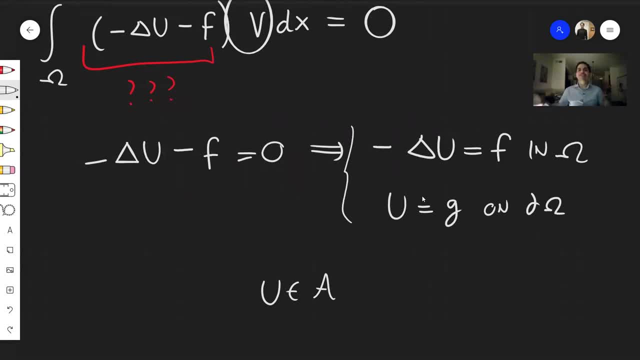 All right, so that was the first part. Again, very classical. the derivation of the Euler Lagrange equation goes the same. but let me also quickly prove the other part, since this is very fun actually. So suppose now that U solves. so minus Laplacian of U equals F. 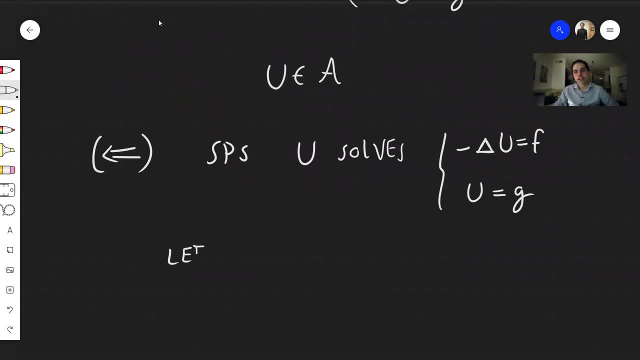 and then U equals G on the boundary and let V in our admissible class- so V is smooth and equal to G on the boundary- be arbitrary, Or yeah, let's say its be arbitrary. And what we want to show essentially is that ar minimizes the energy. 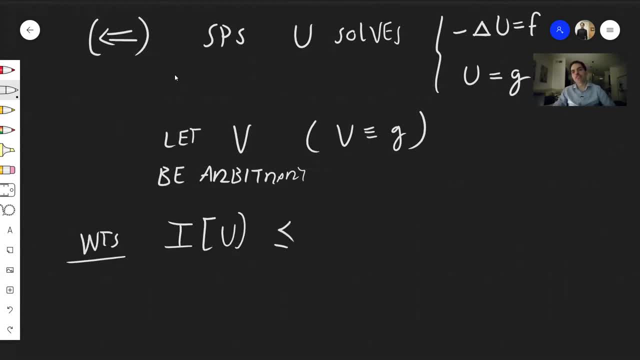 So what we want to show is that I of U is less than or equal to I of V. So no matter which function we pick, you mean the energy at U is smaller than the energy of V. This means minimization. And here's a cool trick: consider Poisson's equation. 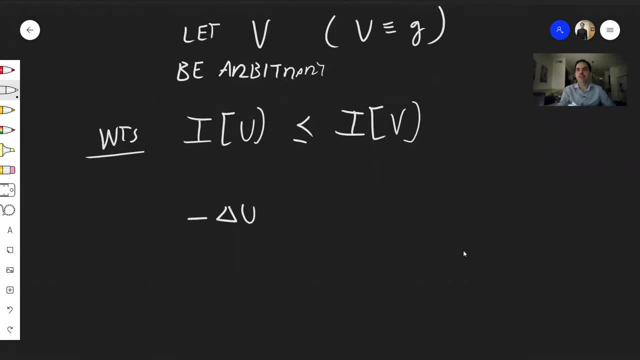 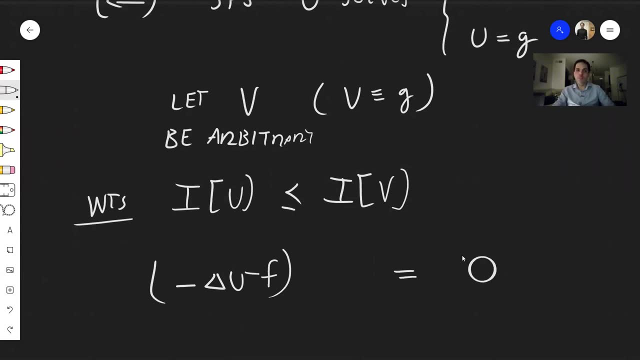 why? Why is Poisson's equation is less than or equal to L equation. so minus Laplacian of u, let's say minus f. On the one hand this equals zero, On the other hand. well, let's take this equation and multiply it by u minus v. 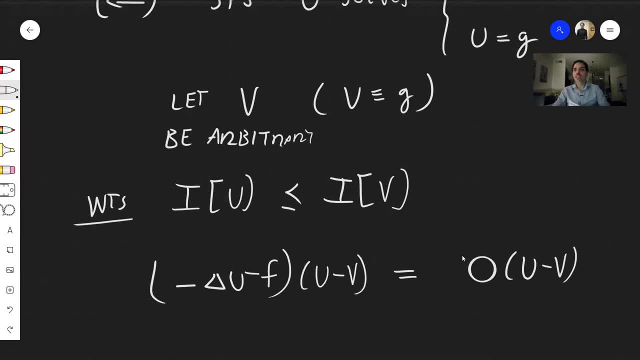 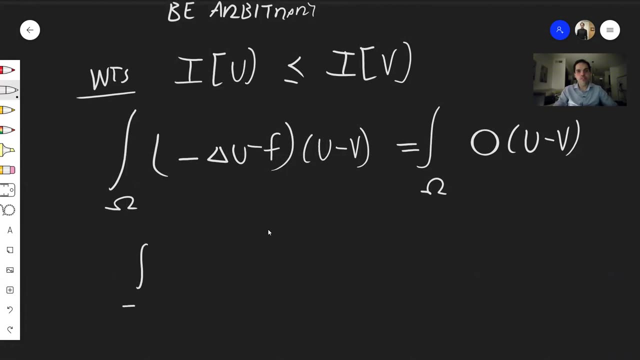 Why are we doing that? Because u minus v is actually zero on the boundary. So let's take that and integrate over our domain. Then, on the one hand, what we get is that this thing equals zero, So integral of over omega, if you want, of minus Laplacian u times. u minus v minus f times. 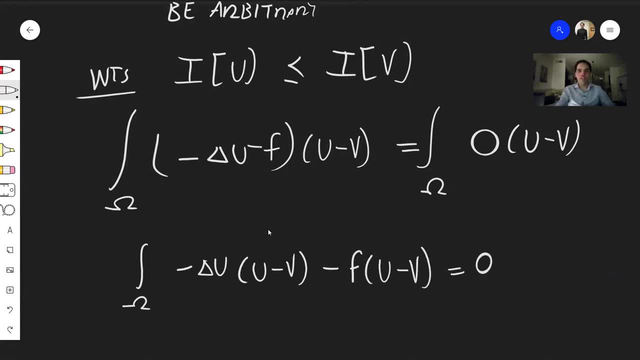 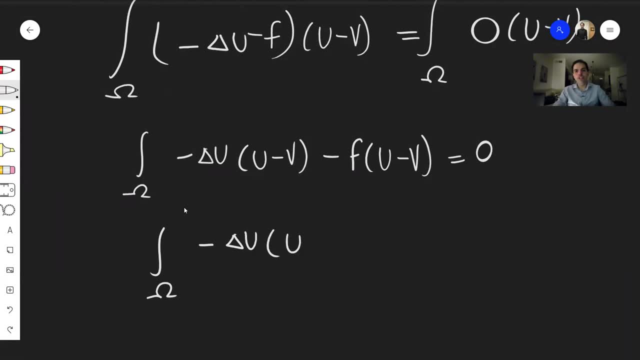 u minus v equals zero And which, if you want, you can just write as integral over omega of minus v. Laplacian: u u minus v equals f times u minus v. But now because again we want to turn this: 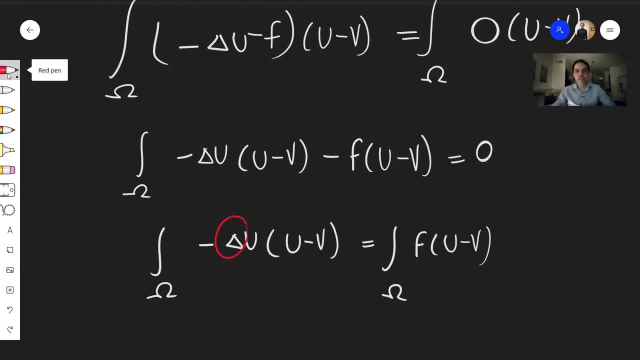 into derivatives. let's just integrate by parts. Again, there might be boundary terms, but not here, because remember, on the boundary, u minus v is just g minus g and that's zero on the boundary, So 0. When it's integrating by parts, you don't have to worry about boundary terms, And then what you get. 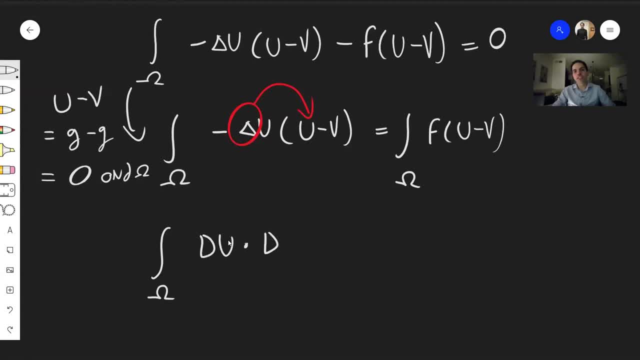 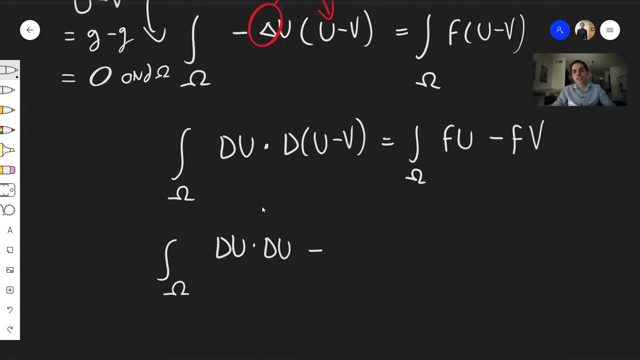 is basically: du dotted with du minus v equals again integral of fu minus fv, And this just becomes, if you expand it out, integral of du dotted with du minus du dotted with dv. All right, Good, So ideally what we would like to do: let's put all the u's on one side. 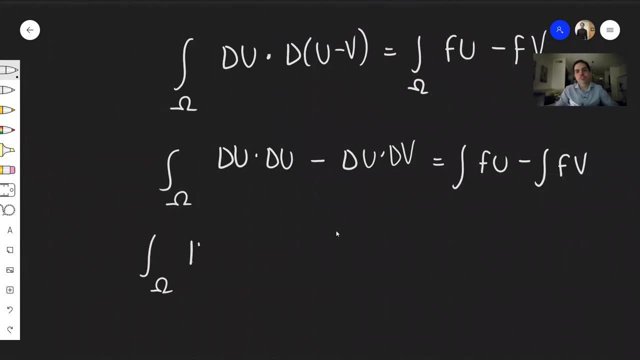 all the v's on the other side. So we get integral of du squared. And then let's put fu here. So minus fu equals integral of du dotted with dv minus fv. Now this is good, Except there are two issues. On the one hand, in our functional there was this 1 half, So it almost. 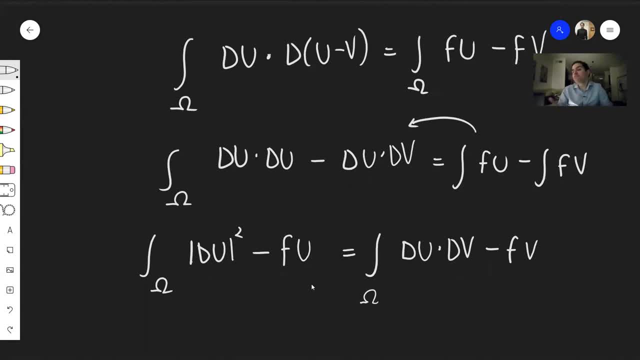 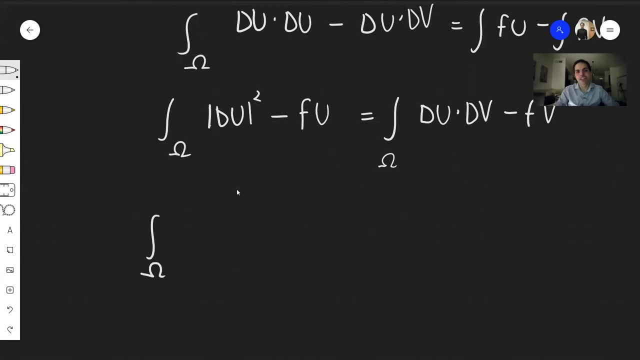 looks like our functional, On the other hand. well, here we have u and v. Ideally, we just want to have v, And the way to solve this it was with the following clever trick: So take this du dotted with dv. Well, a function, a scalar function, here it's always less than or equal to its 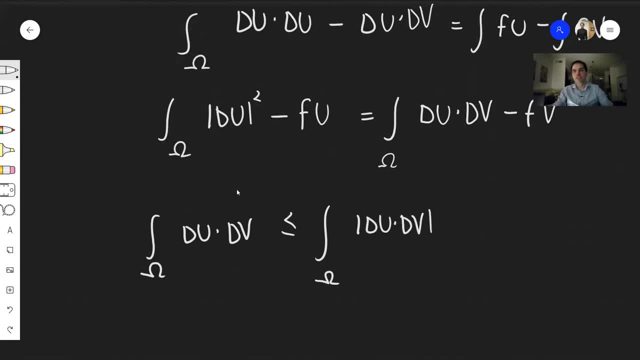 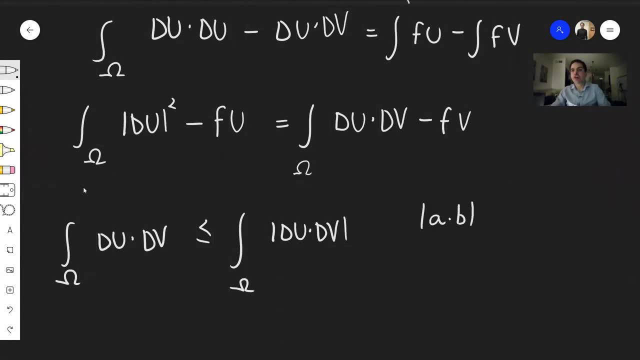 absolute value. Now, here we have absolute value of a dot product, which should remind you of the Cauchy-Schwarz inequality or Cauchy-Schwarz-Bunyakov scheme, which says that the magnitude of the dot product 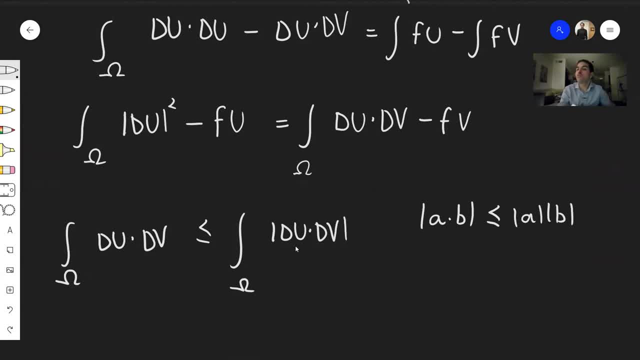 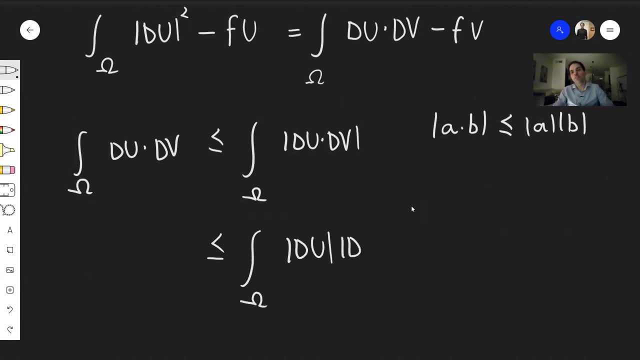 is less than or equal to the magnitude of those two vectors. So, in particular, what we get this is less than or equal to du times dv. Again, this means that the magnitude of the dot product is less than or equal to this norm. And, moreover, 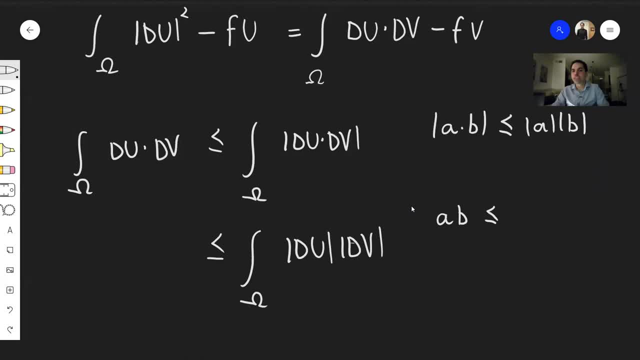 we have to use another equality, called Cauchy's inequality, which simply says ab is less than or equal to 1 half a squared plus 1 half b squared, which you can simply prove because a minus b squared is greater or equal to 0.. Expand that out and solve for ab and you get. 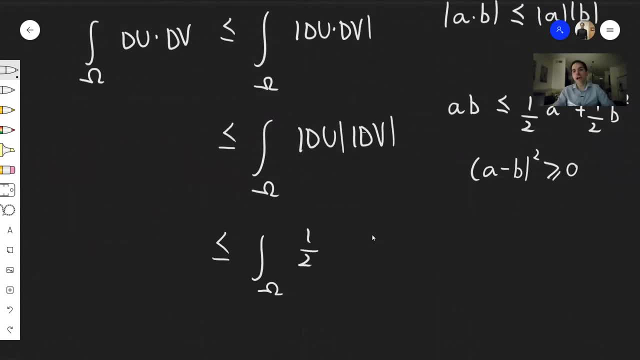 this thing. So in this problem, what this becomes is integral of 1 half du squared plus 1 half dv squared, And it's good to isolate. you know, like here, it's very good if you're dealing with products, because now, Instead of having du and dv entangled you. 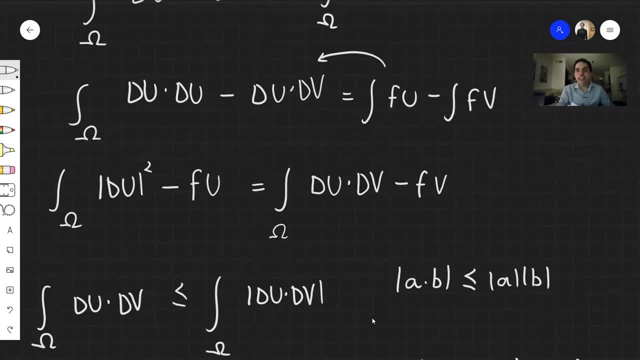 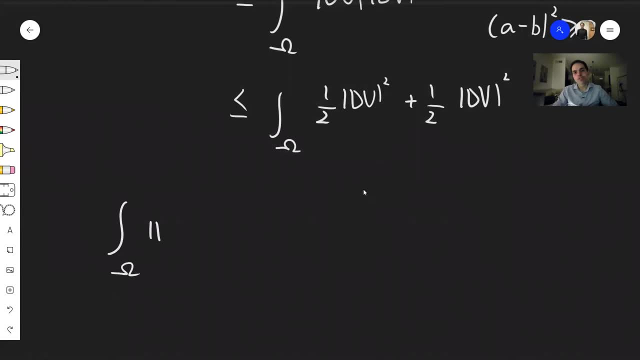 can just separate them out. All right, Very good. And why is this useful? So let's come back to this thing here. So we had integral of du squared minus fu- I'll stop with the cursing a second- And so we get du dotted with dv minus integral of fv. But now we found that this thing 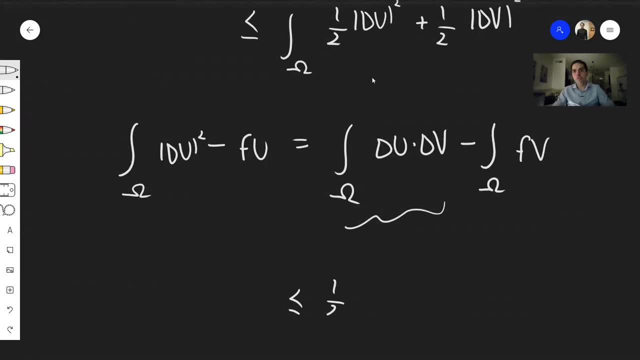 is less than or equal to one half. Well, yeah, it is one half du squared plus one half dv squared minus fv. All right, And again, this is du squared minus fu. All right, And then we're almost done. So here's a cool thing. And again it's almost magic, Those energy methods, it's always like. 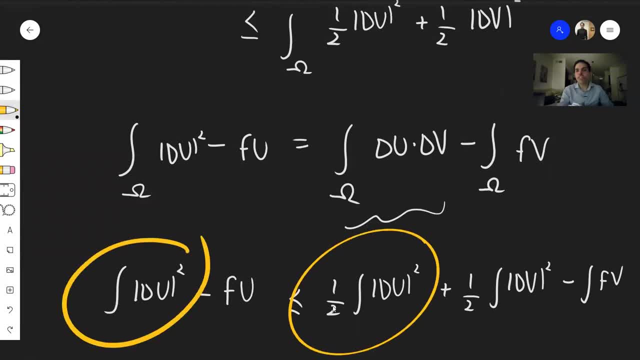 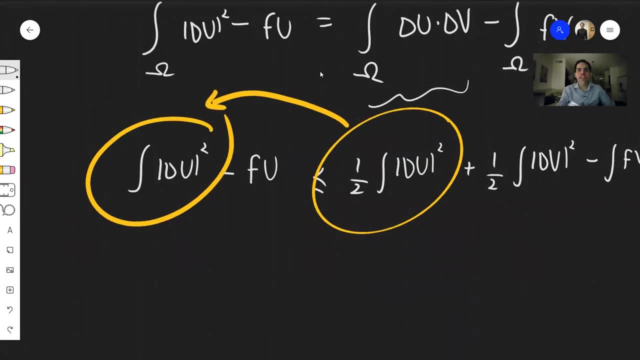 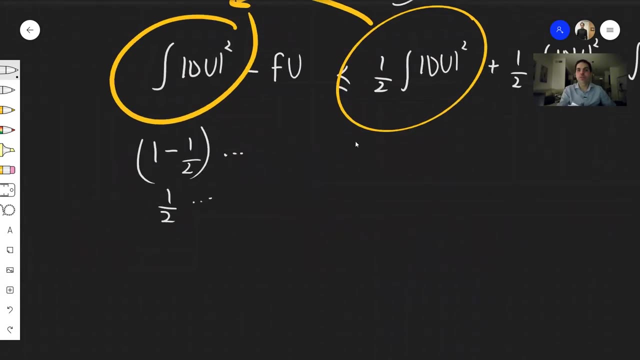 magic here, Because here we have du squared, Here we have one half du squared. If you put this here, I don't know why it's so thick, but you basically get one minus one half of that, Which is just one half of this. So, in the end, what you get is indeed so integral.